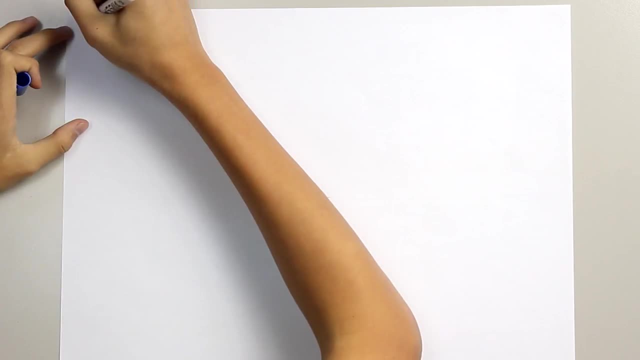 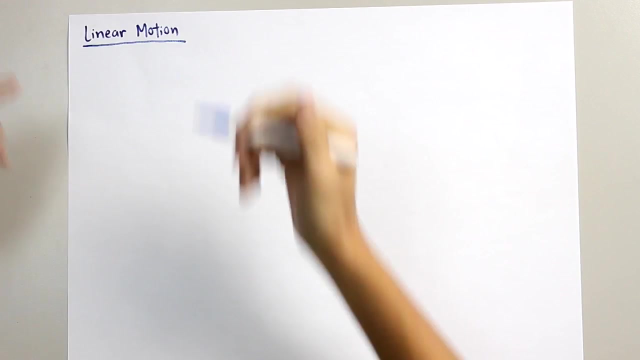 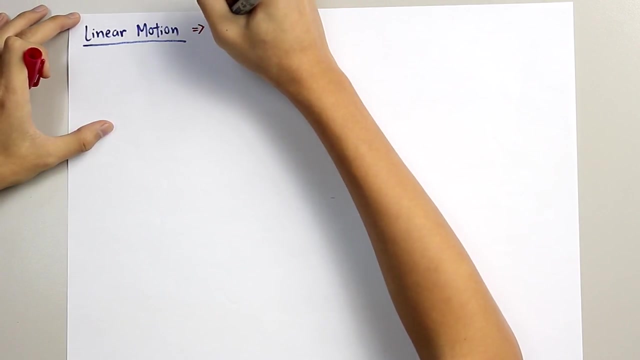 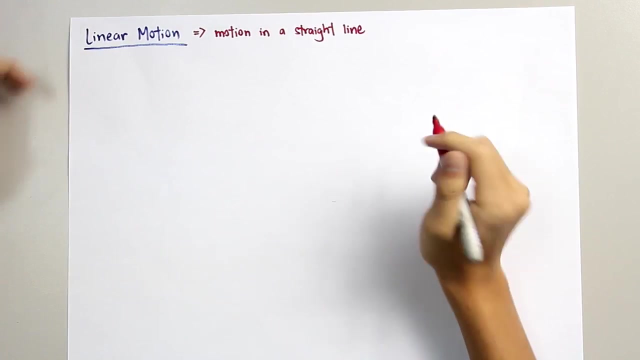 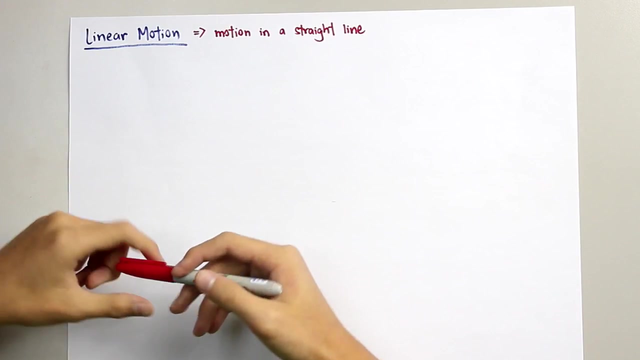 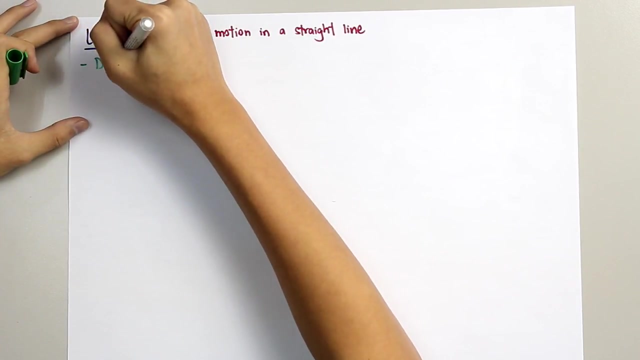 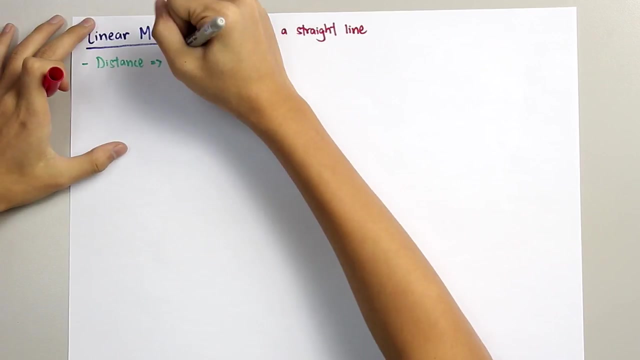 Hello again. For this lesson we will learn linear motion. Linear motion is the motion in a straight line. Let's start from the introduction of distance, displacement, speed and velocity. First, distance: Distance is defined as. distance is defined as the total length of path. 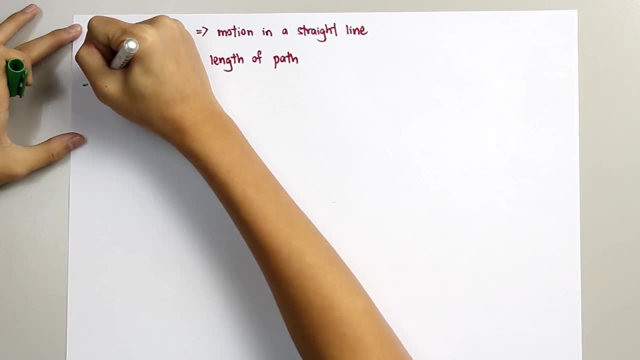 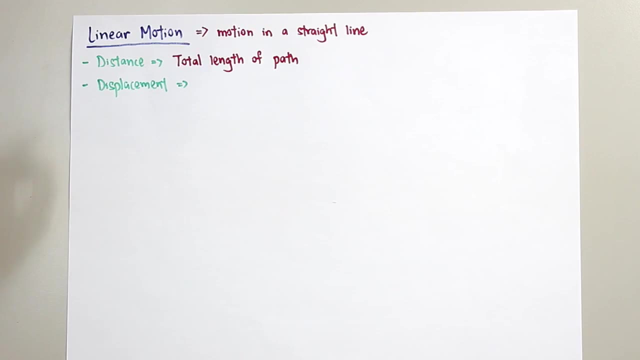 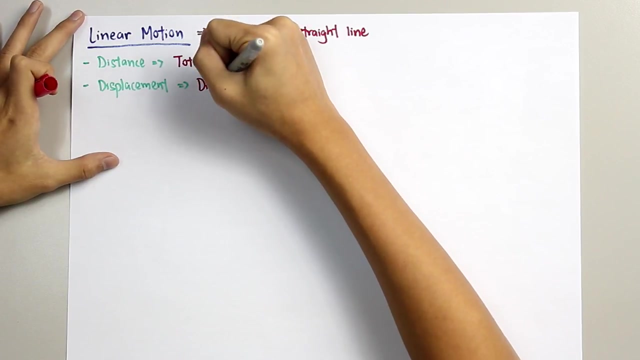 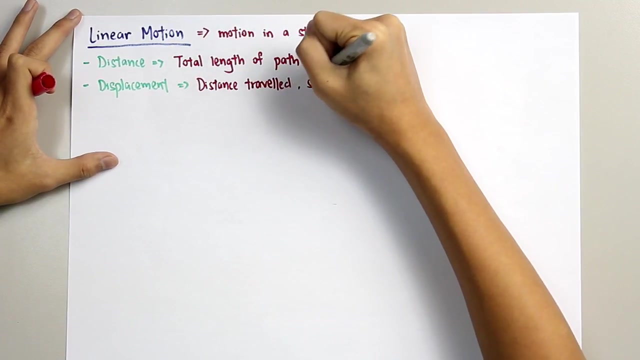 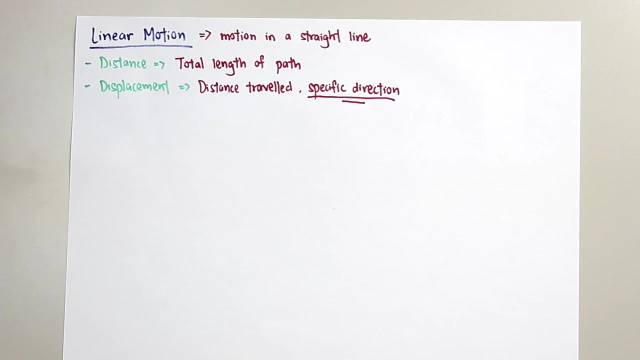 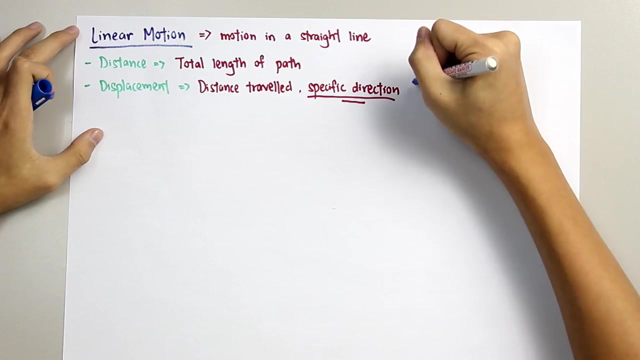 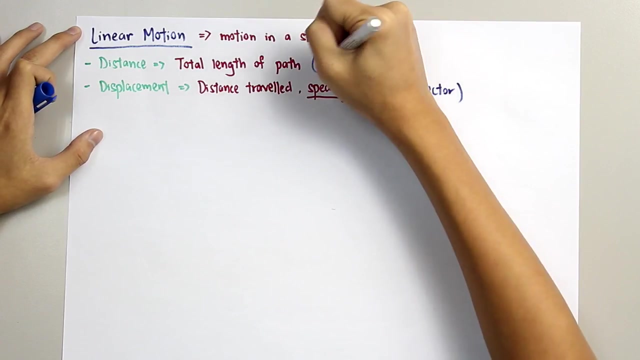 Second, displacement. The definition for displacement is the distance travelled in a specific direction, And we know that scalar is a quantity that only has magnitude, whereas vector is a quantity that has magnitude and direction. So displacement is a vector quantity And whereas 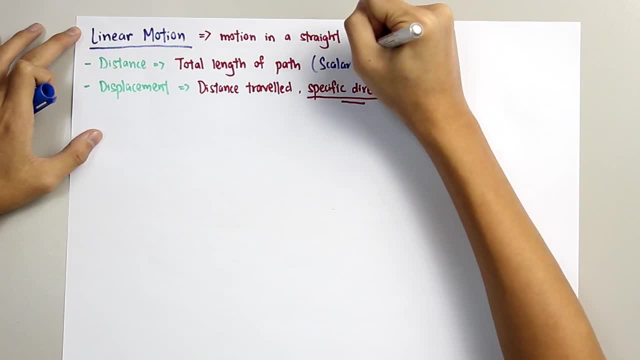 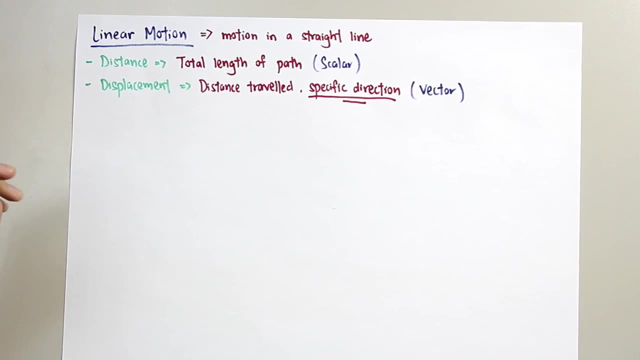 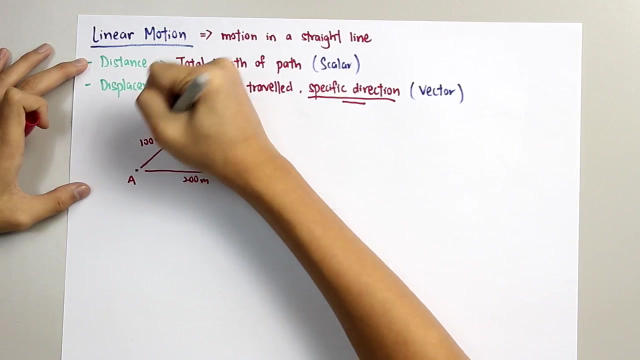 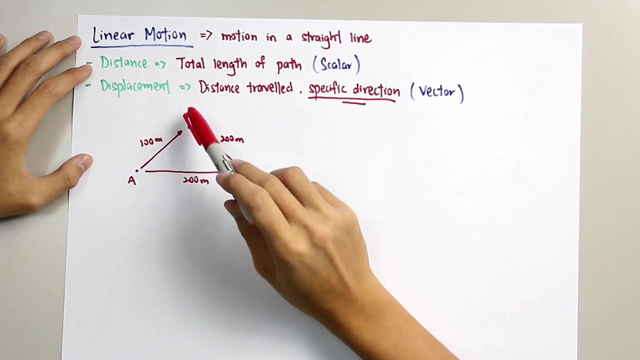 distance is a scalar, since the direction is not important. Now I'll show you some examples to differentiate distance and displacement. Given a city A, a city B and a city C, a driver needs to travel from city A to city C, So the driver takes the route from A to B and B to C. 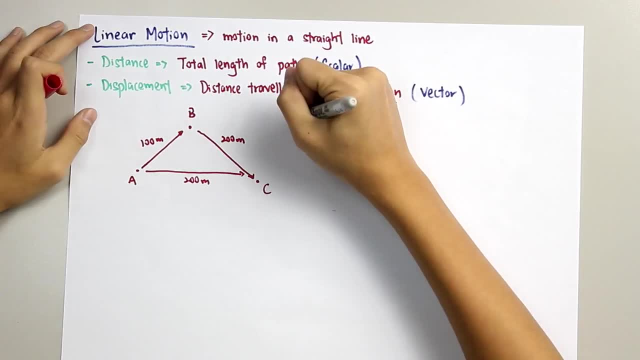 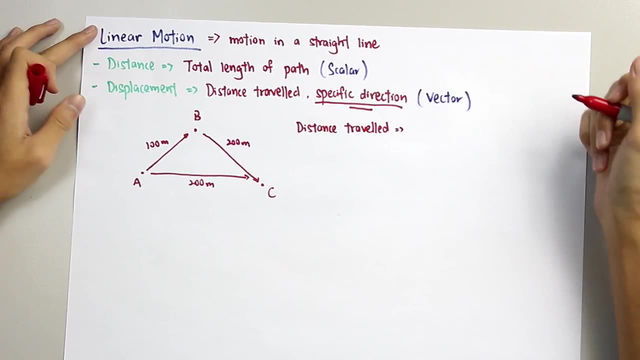 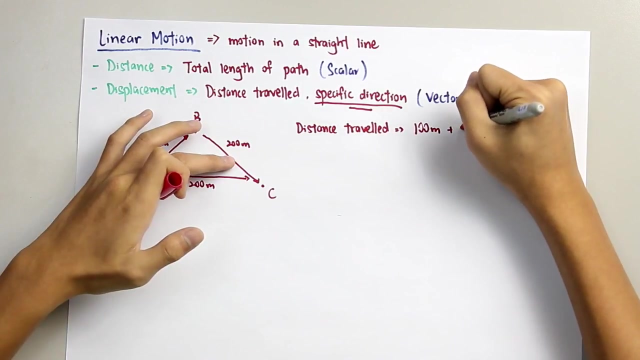 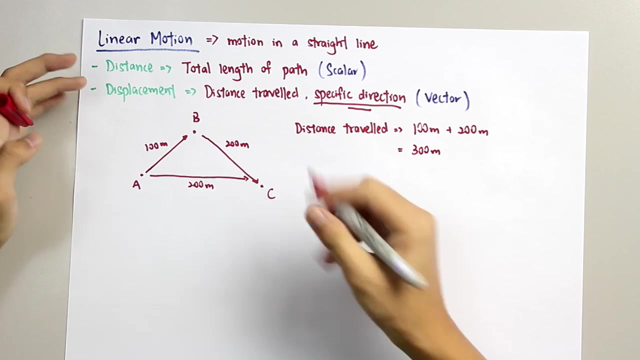 And so the distance travelled, distance travelled, distance travelled and the distance travelled, The distance travelled by the driver, is one hundred meter plus two hundred meter equals to three hundred meter, equals to three hundred meter. However, for this placement we mentioned, that is a distance travelled. 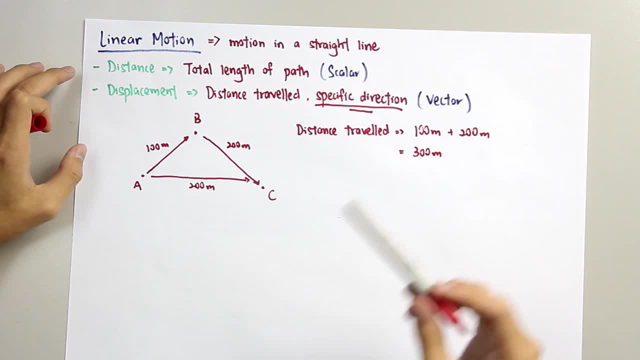 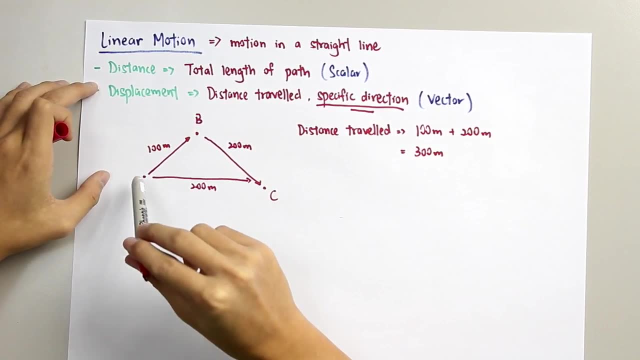 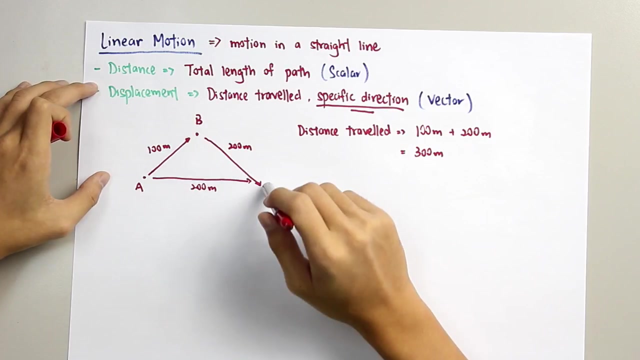 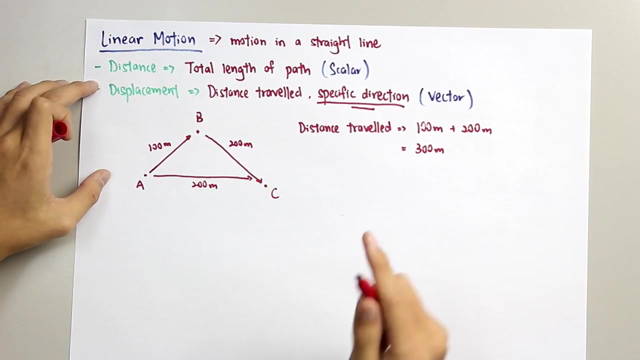 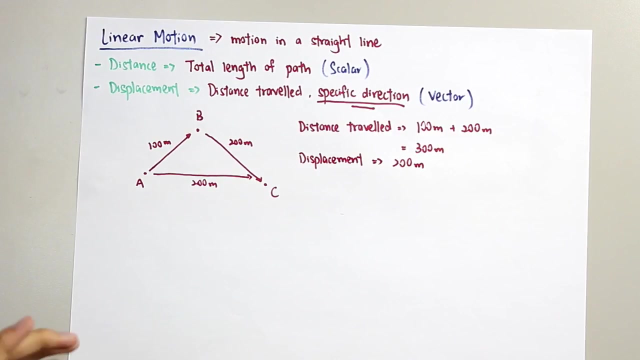 in a specific direction, which means that when you need to calculate the displacement travelled, you have to give only this direction, only one direction. if you give A to B and B to C, the definition is not valid, since there are two direction. so the displacement is 200 meter. next, speed and velocity. 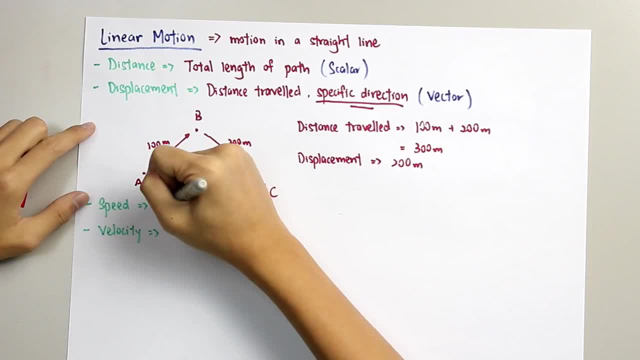 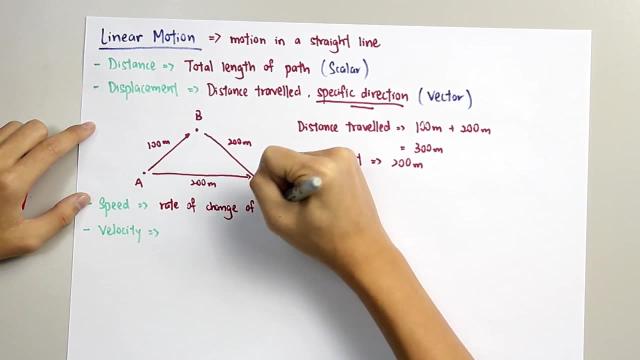 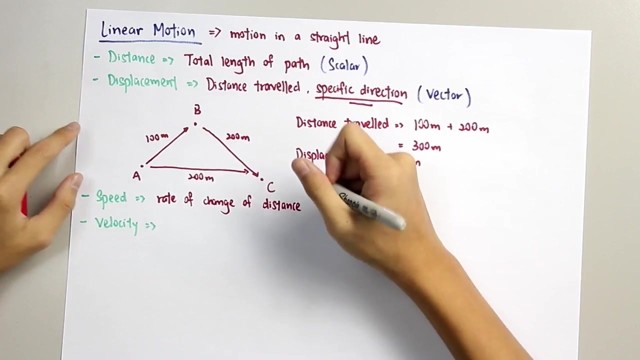 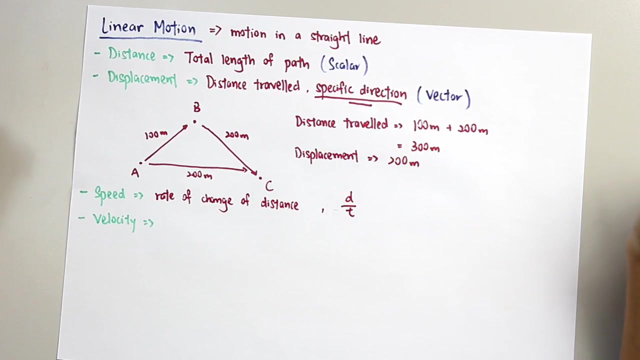 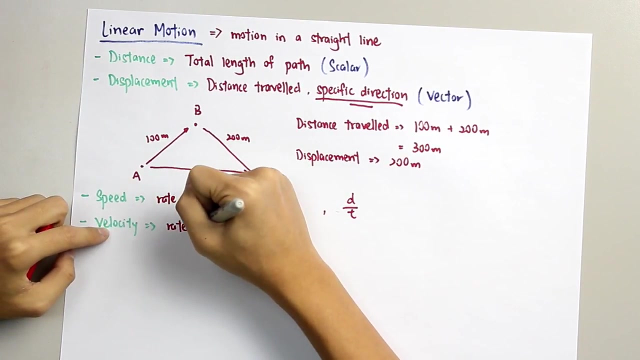 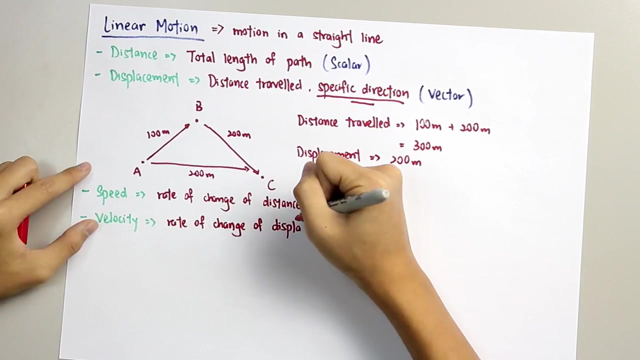 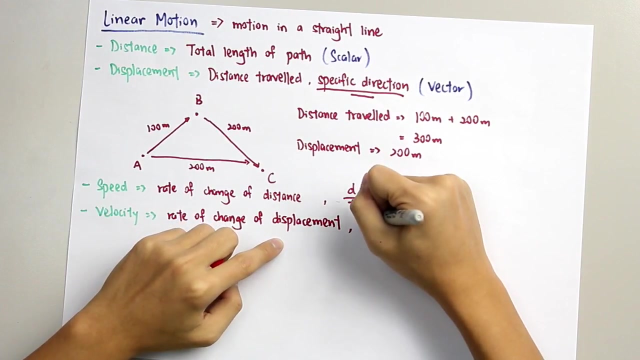 speed is the rate of change of distance and since we say that is a rate of change of distance, so the formula for speed is the distance over time, whereas for velocity it is the rate of change of displacement, and for the formula is the displacement represented by the letters S over the. 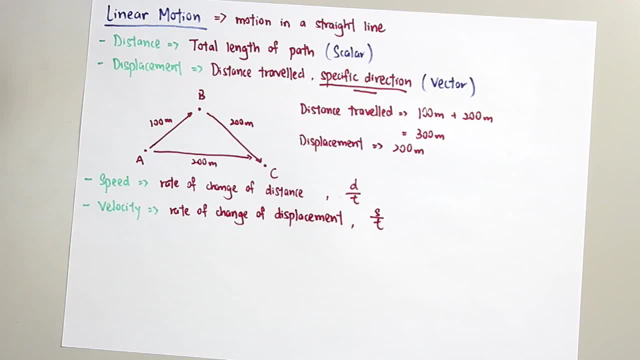 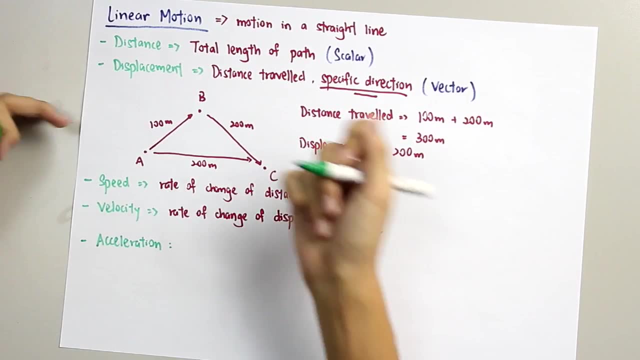 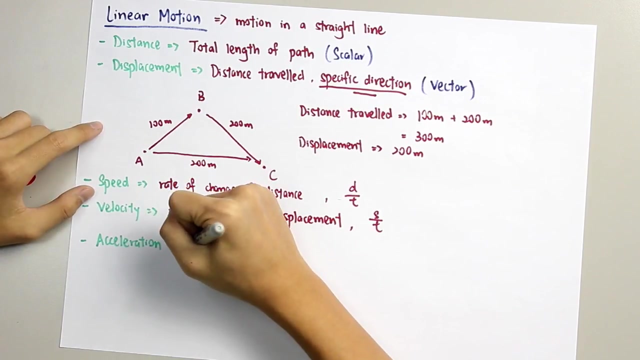 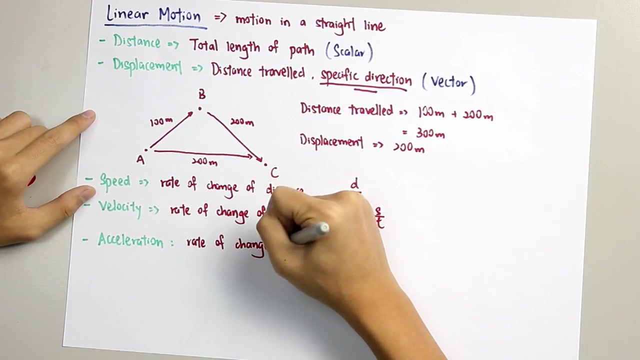 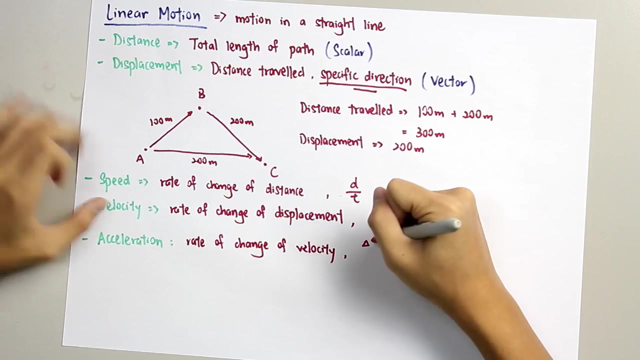 time. so next, what is acceleration? we know that when a car is going faster and faster and faster, the car experiences acceleration. therefore, we give the definition of acceleration as rate of change of velocity and formula: change of velocity V over time. or you can write it as the final velocity V over time. 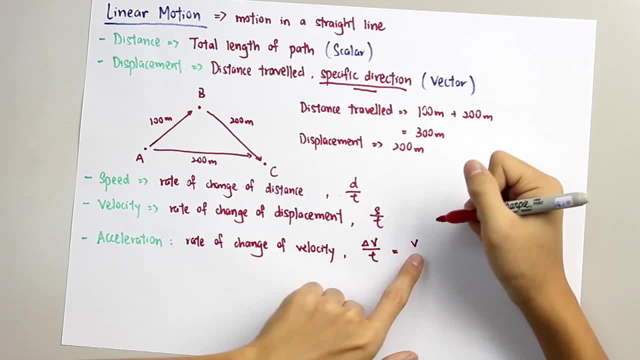 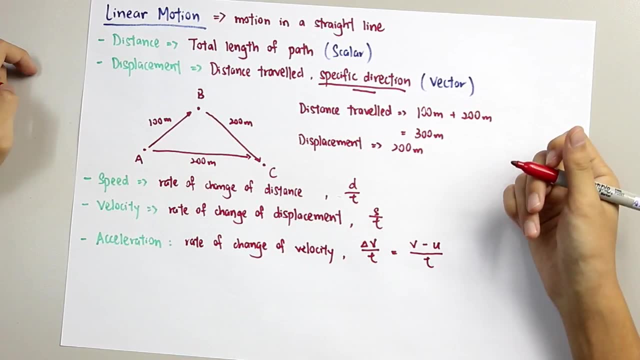 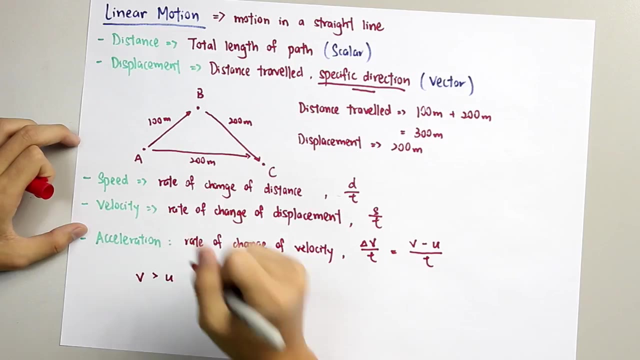 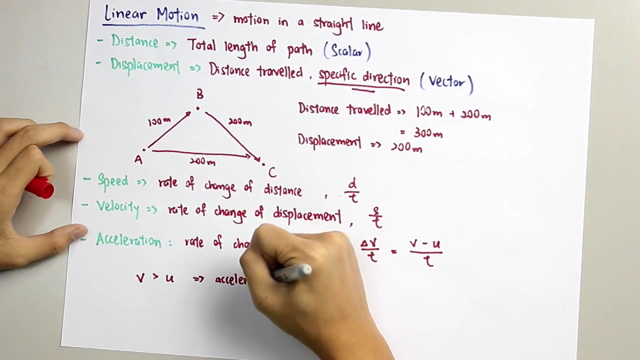 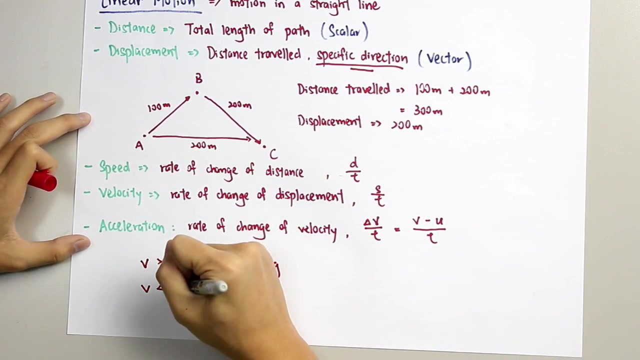 or you can write it as the final velocity V over time minus initial velocity u over time. So when v, the final velocity is greater than u, we can say that the object is accelerating, And when v, the final velocity is lesser than initial velocity.